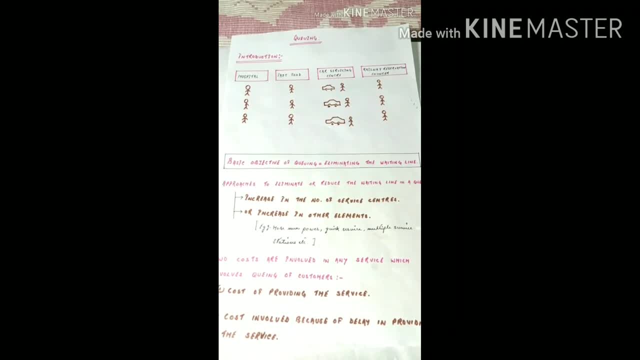 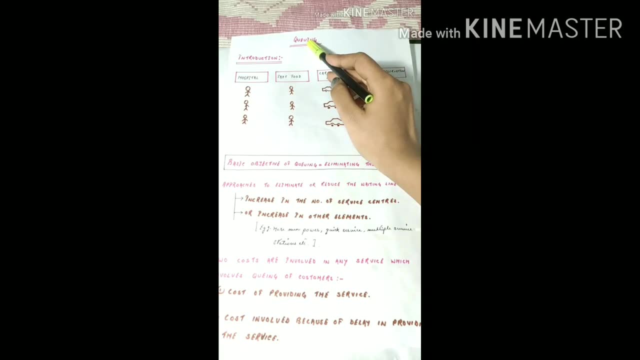 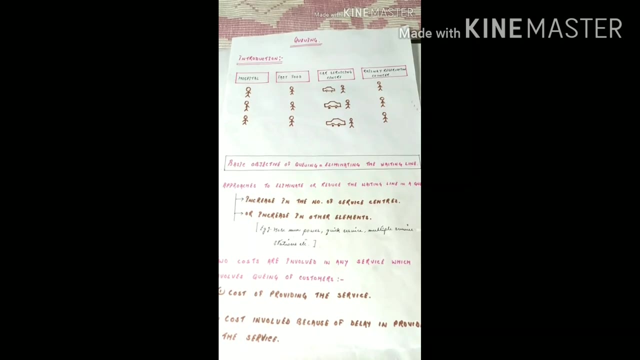 to cover a very simple as well as a very important topic relevant to management as well as engineering studies. So, yeah, that is queuing, as I have written here. So I guess many of us has come across this topic. under the subject operation features either be in: 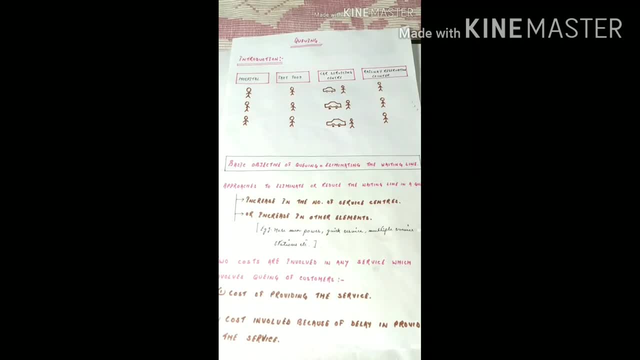 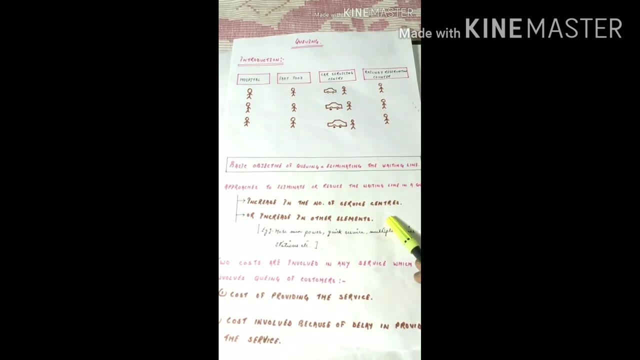 management or in engineering. So we are trying to give an overview of what queuing is and what are the elements under queuing and what are the key processes, including consumer behavior and various other factors. So the basic idea is that the number of service centers 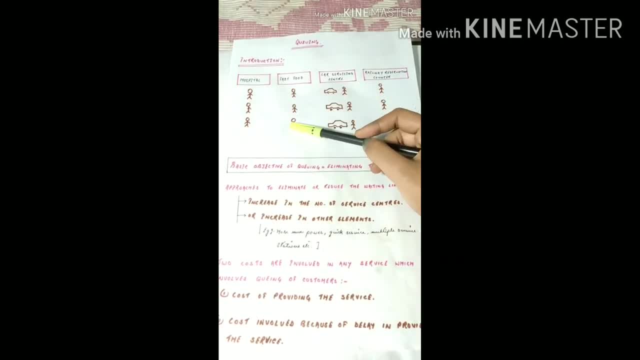 is quite less as compared to customers waiting in the service centers. So, then, there is no other option than to wait in a queue, because that is the only civilized way of getting a service, and that too, without indulging in any fights or without indulging in any conflicts. 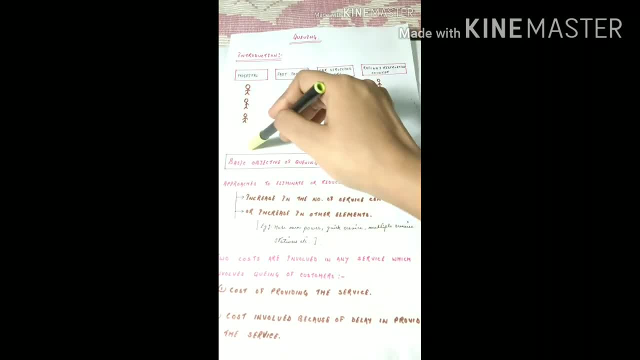 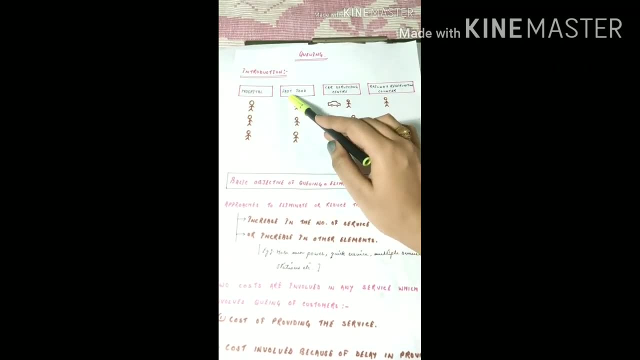 So, as you can see, I have drawn a diagram to make you understand the saying. So the first thing I am going to do is I am going to draw a diagram to make you understand the saying. So I have taken four examples: A hospital, a fast food, a car servicing center, a railway. 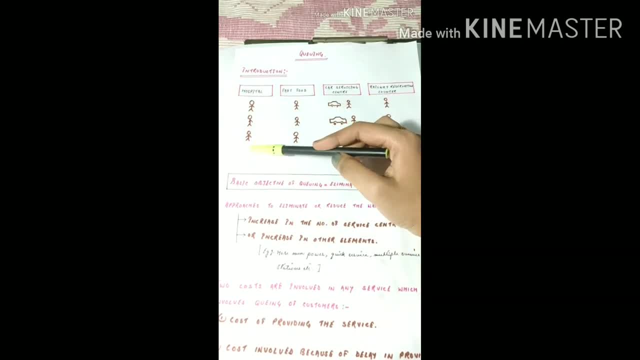 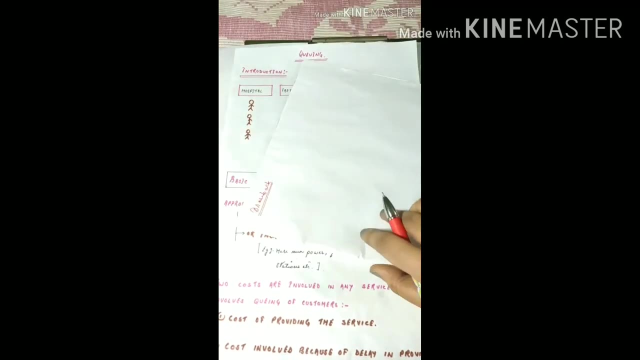 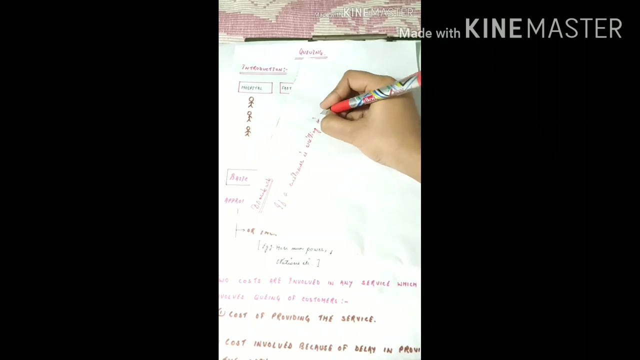 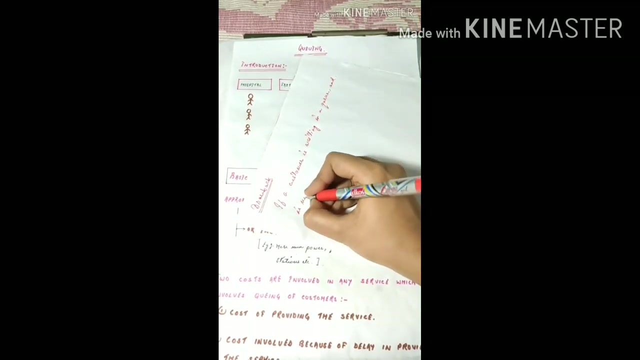 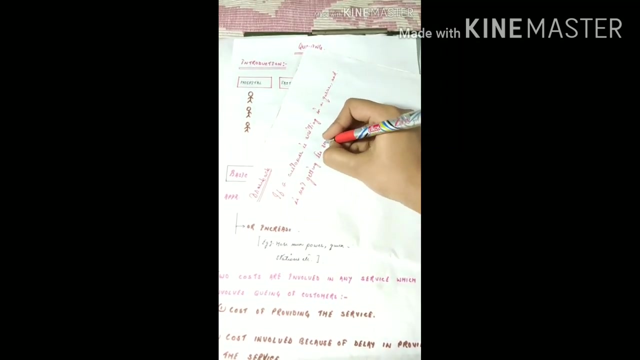 reservation counter, You can see people are waiting or maintaining queue to get their services accordingly. But this concept, too, has a drawback. So what is the drawback? and we will discuss about the drawback. The drawback is that If a customer is waiting in a queue and is not getting the service, So this concept is 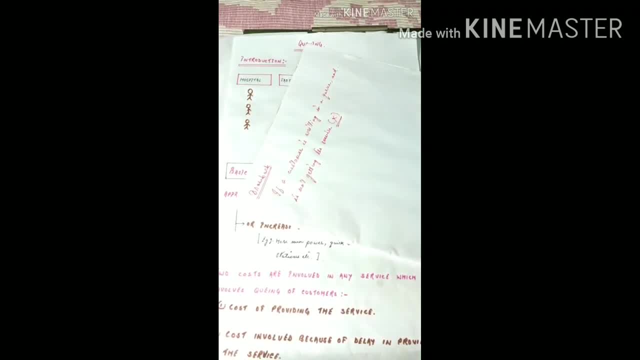 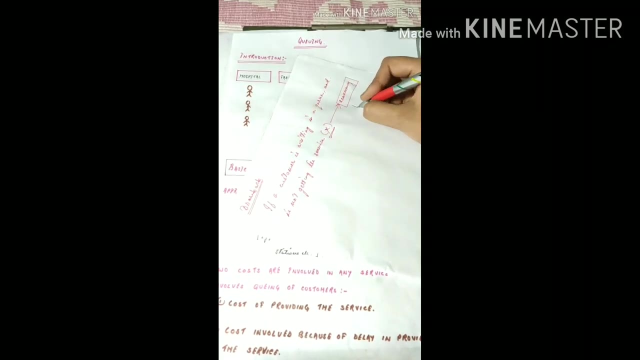 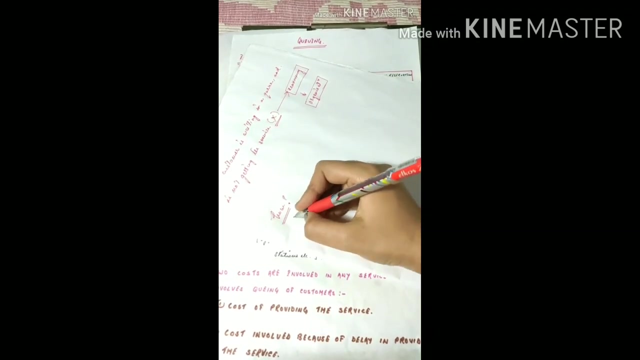 boring and is not, is not expected by the customer. so this will directly impact the economy of the organization. yeah, so this concept will directly impact on the economy of the organization and how. we will also see how to answer this. the customer always things, always things of alternative, alternative, that is, this alternative is: what that is. other service center, other service center where they will get quick service, the same service will be. service center where they will get quick service, the same service will be service center where they will get quick service, the same service will be provided in a short amount of time. so 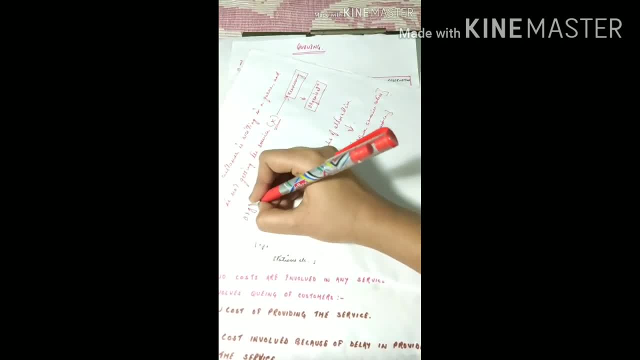 provided in a short amount of time. so provided in a short amount of time. so the customer will move from this, the customer will move from this. the customer will move from this organization- the first organization- to organization, the first organization to organization, the first organization to the second organization. and when this 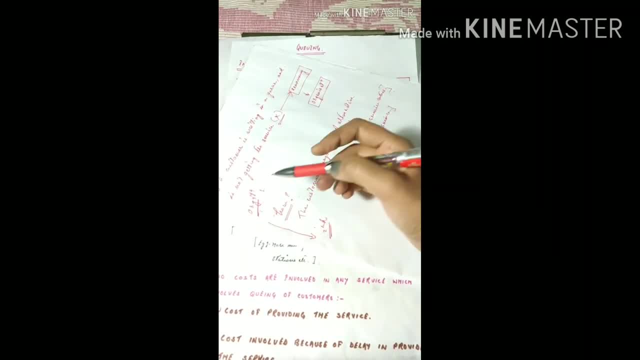 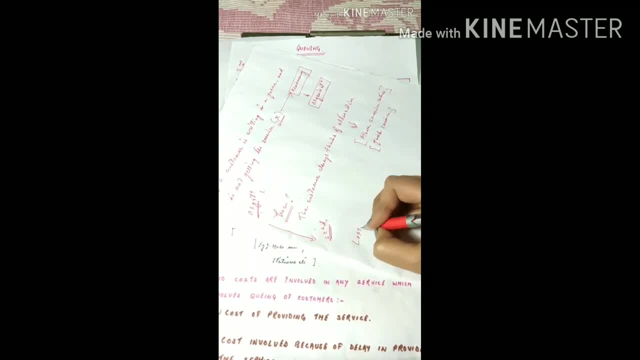 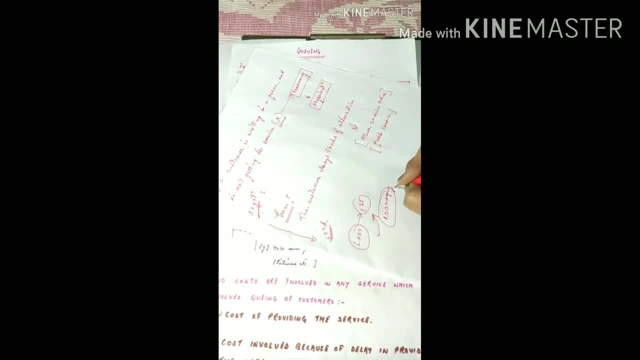 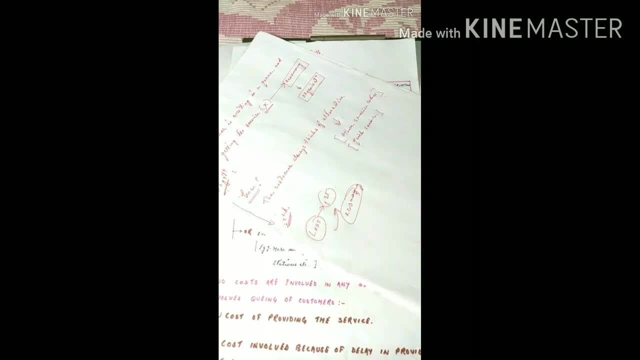 impacts on the economy of the first, impacts on the economy of the first organization. it called norm media, sorry organization. it called norm media, sorry organization. it called norm media, sorry. so, now that we know the introduction, now, so, now that we know the introduction, now, so now that we know the introduction, now that we know the introduction, we can. 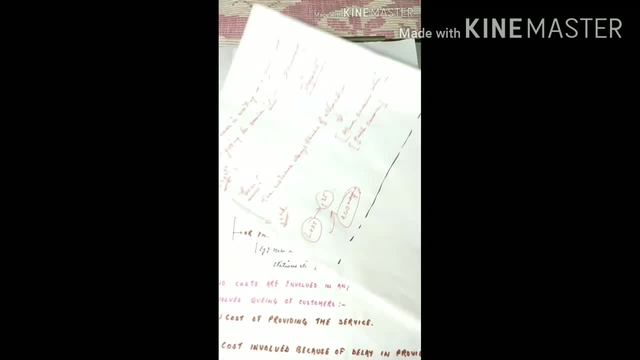 that we know the introduction. we can, that we know the introduction, we can move on to the objectives, move on to the objectives, move on to the objectives. so what is the objective of queuing? so what is the objective of queuing? so what is the objective of queuing theory? as you can see, here I have written. 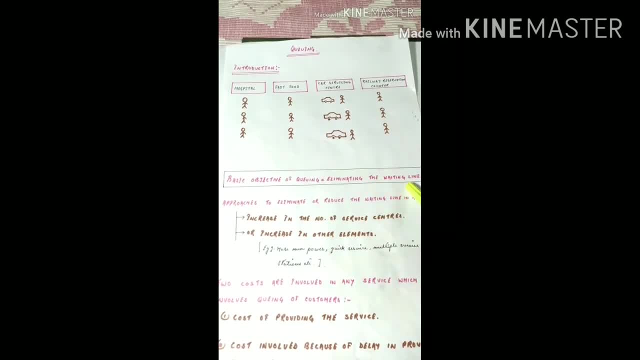 theory. as you can see here I have written theory. as you can see here I have written. basic objective of queuing is eliminating. basic objective of queuing is eliminating. basic objective of queuing is eliminating the waiting time. so the main objective, the waiting time, so the main objective. 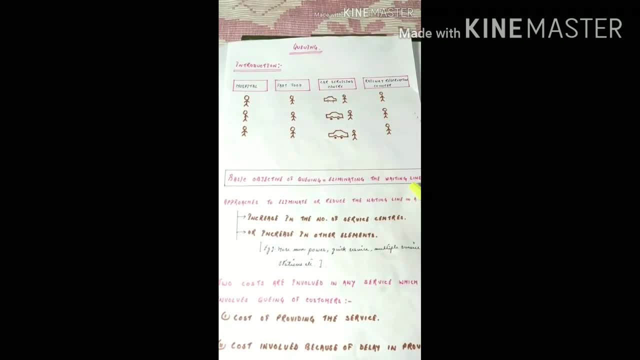 the waiting time. so the main objective will be to eliminate the waiting line. so will be to eliminate the waiting line. so will be to eliminate the waiting line. so how do we eliminate the waiting line now? how do we eliminate the waiting line now? how do we eliminate the waiting line now? we have two approaches to reduce the 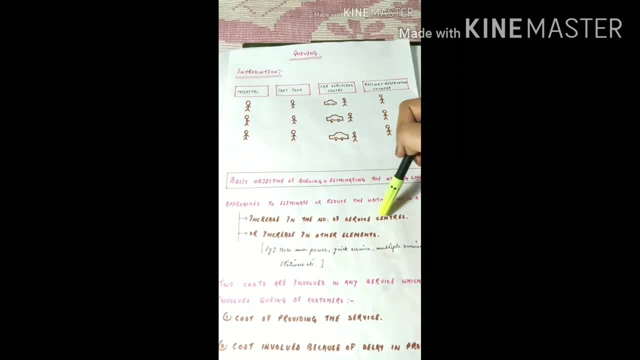 we have two approaches to reduce the. we have two approaches to reduce the waiting line. that is the first is waiting line. that is the first is waiting line. that is the first is increase in the number of service centers. increase in the number of service centers. increase in the number of service centers. either we will have to increase the. 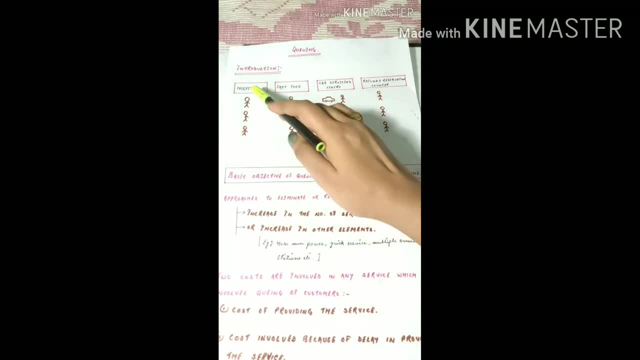 either we will have to increase the, either we will have to increase the number of service centers. that is, let us number of service centers. that is, let us number of service centers. that is, let us take the example of the hospital. if we take the example of the hospital, if we 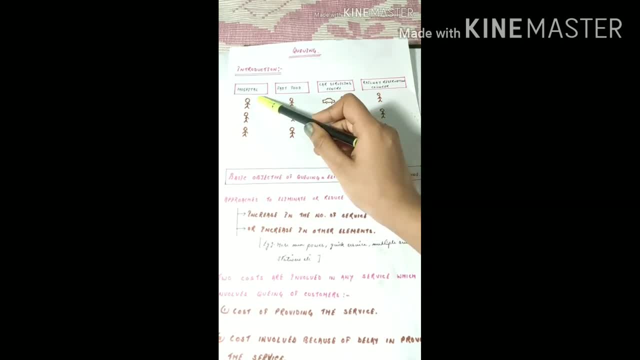 take the example of the hospital. if we take the example of the hospital, then if take the example of the hospital, then if take the example of the hospital, then if previously there were one reception, previously there were one reception, previously there were one reception counter, then we will have to increase the. 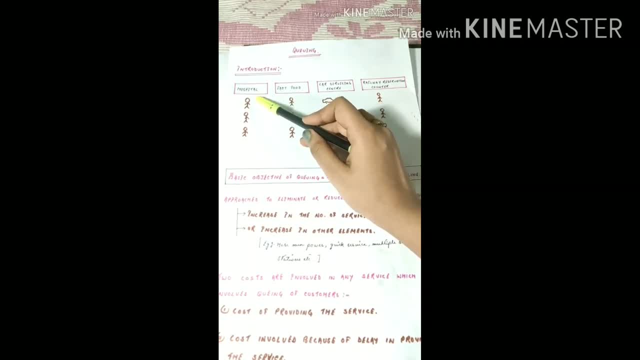 counter, then we will have to increase the counter, then we will have to increase the reception centers, maybe two, three or reception centers, maybe two, three or reception centers, maybe two, three or likewise. and that is the first case and likewise, and that is the first case. and secondly, it says increase in other. 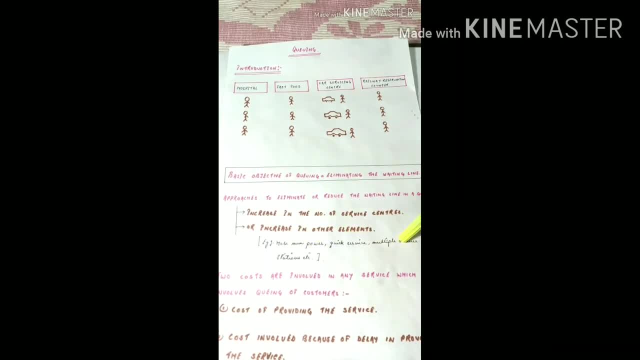 secondly, it says increase in other. secondly, it says increase in other elements, for example more manpower, quick elements. for example: more manpower, quick elements. for example more manpower, quick service, multiple service station, etc. so service, multiple service station, etc. so service, multiple service station, etc. so yeah, more manpower means, if we are not 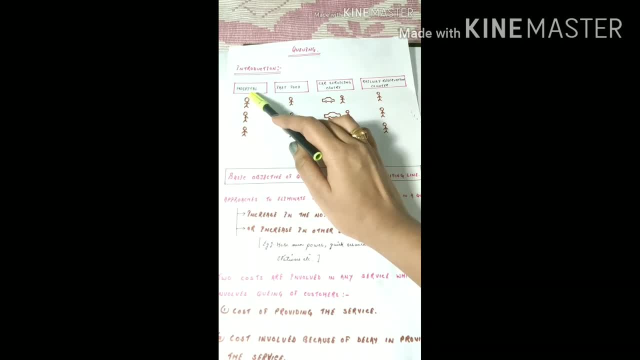 yeah, more manpower means if we are not, yeah, more manpower means if we are not increasing the reception centers in a, increasing the reception centers in a increasing the reception centers in a hospital, then what we will have to do is hospital. then what we will have to do is: 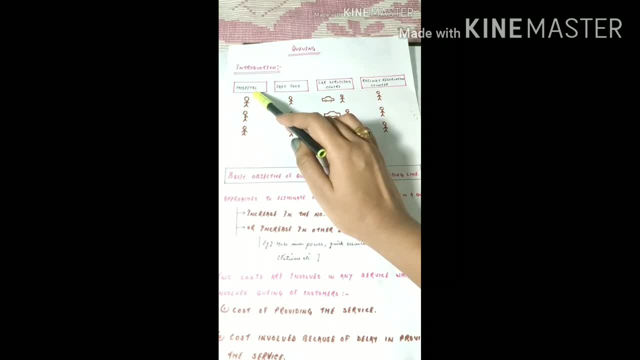 hospital, then what we will have to do is that in the same reception counter will that in the same reception counter, will that in the same reception counter will we will have to induce more manpower, we will have to induce more manpower, we will have to induce more manpower. that is, we will have to induce more. 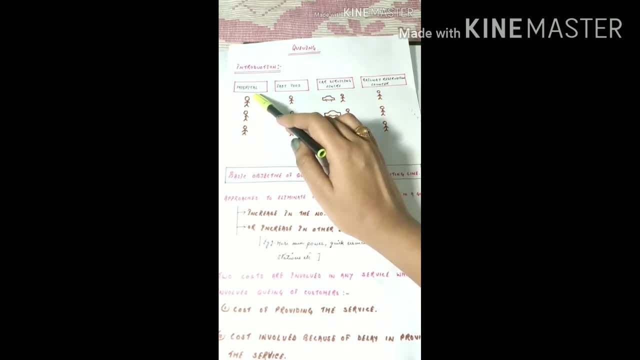 that is, we will have to induce more. that is, we will have to induce more people to serve as receptionist, so that people to serve as receptionist, so that people to serve as receptionist, so that people get services quickly- okay, now we. people get services quickly. okay, now we. 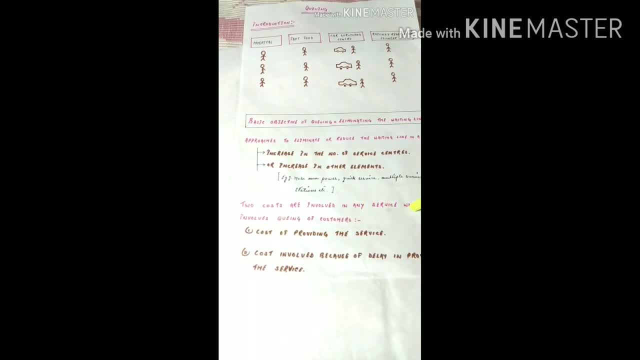 people get services quickly. okay, now we have the cost to cost or involving any, have the cost to cost or involving any, have the cost to cost or involving any service which involves queuing of service, which involves queuing of service which involves queuing of customers. so, while we go for the cost, we 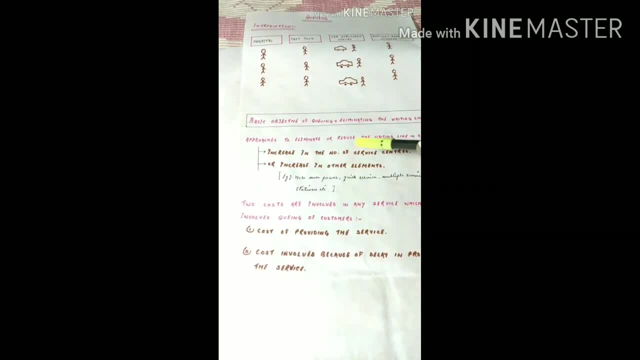 customers. so while we go for the cost, we customers. so while we go for the cost we have, the first one is cost of providing have. the first one is cost of providing have. the first one is cost of providing the service that is a company has to, the service that is a company has to. 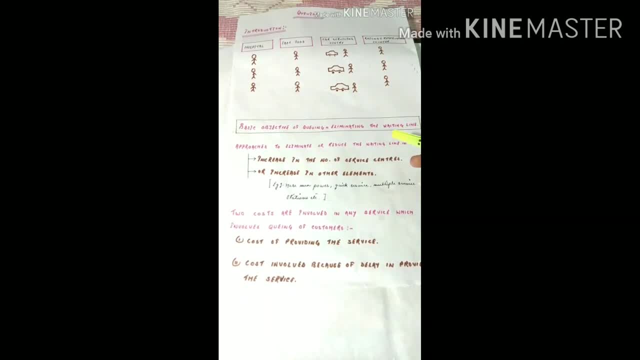 the service, that is, a company, has to invest some amount of their capital in invest some amount of their capital in invest some amount of their capital in providing a particular service to the, providing a particular service to the providing a particular service to the customer, since they cannot provide the. 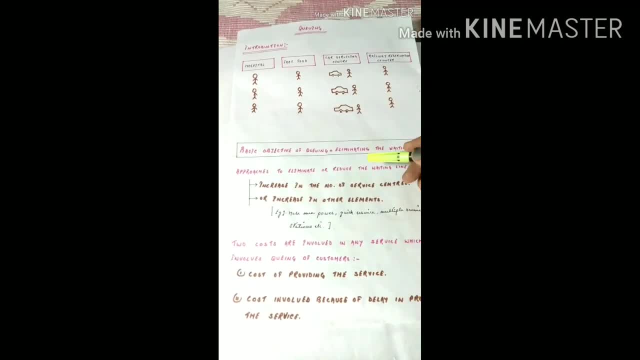 customer, since they cannot provide the customer, since they cannot provide the service for free. so this we can explain: service for free. so this we can explain: service for free. so this we can explain with the help of an example that is in, with the help of an example that is in: 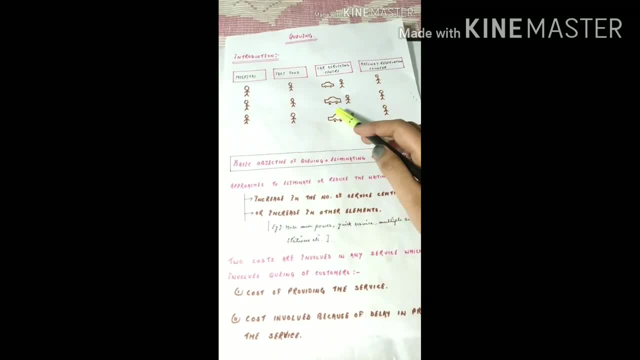 with the help of an example, that is, in case of a car servicing center. if we see case of a car servicing center, if we see case of a car servicing center, if we see a company has to invest some amount of. a company has to invest some amount of. 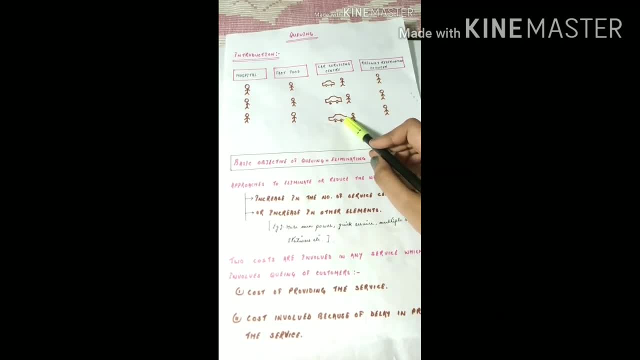 a company has to invest some amount of money in their labors, laborers and other money in their labors laborers and other money in their labors laborers and other name other man machinery equipments. to name other man machinery equipments. to name other man machinery equipments to deliver their services to the customers. 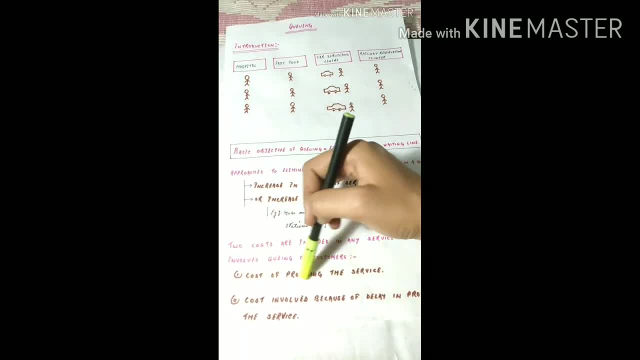 deliver their services to the customers, deliver their services to the customers. so that is that is the cost they are. so that is that is the cost they are. so that is that is the cost they are talking about in the first statement, and talking about in the first statement, and 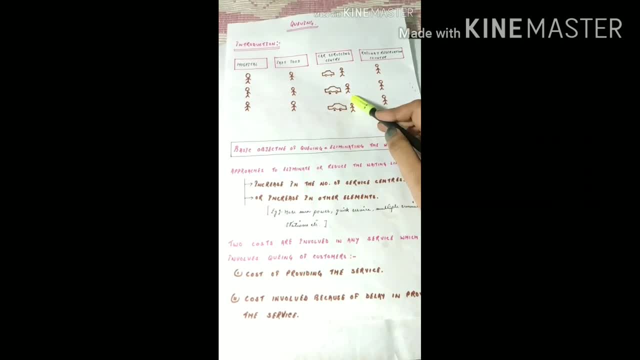 talking about in the first statement and okay, let us take one more example that. okay, let us take one more example that. okay, let us take one more example. that is in case of a fast-food corner. if we is in case of a fast-food corner, if we 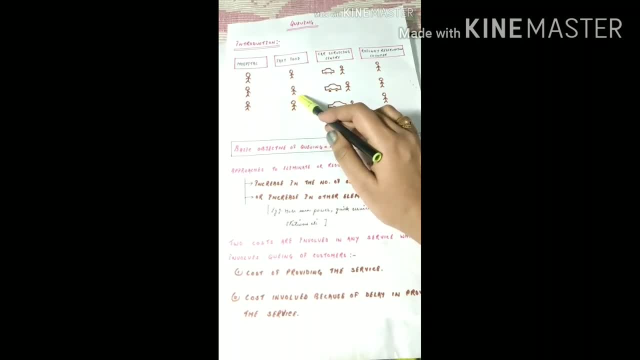 is in case of a fast-food corner. if we see they have to incur the cost of see, they have to incur the cost of see. they have to incur the cost of buying the raw materials and other buying the raw materials and other, buying the raw materials and other materials and provide a prepared food to. 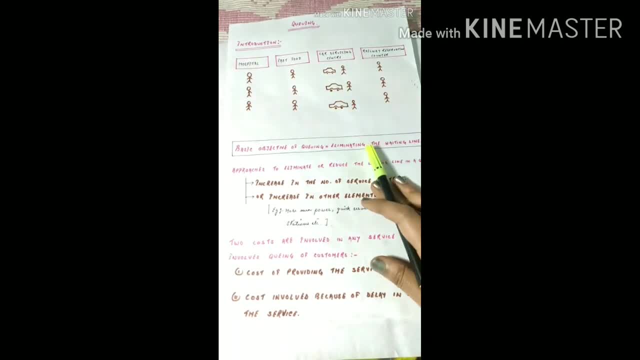 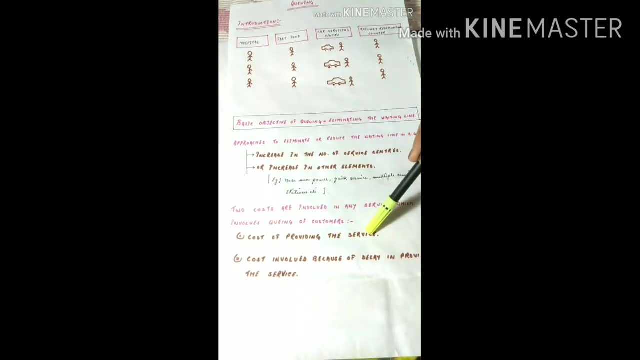 materials and provide a prepared food to materials and provide a prepared food to the customers. so these are the cost the customers. so these are the cost the customers. so these are the cost which the companies or an organization, which the companies or an organization, which the companies or an organization has to incur initially for for this. 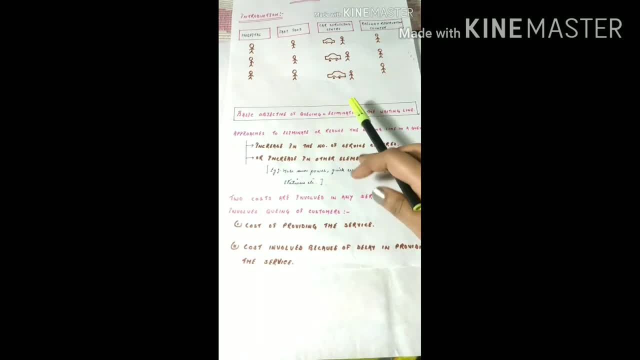 has to incur initially for for this, has to incur initially for for this process. so the next one is: which is process. so the next one is: which is process. so the next one is: which is highlighted: is cost involved. between highlighted: is cost involved. between highlighted: is cost involved. between cost involved because of delay in 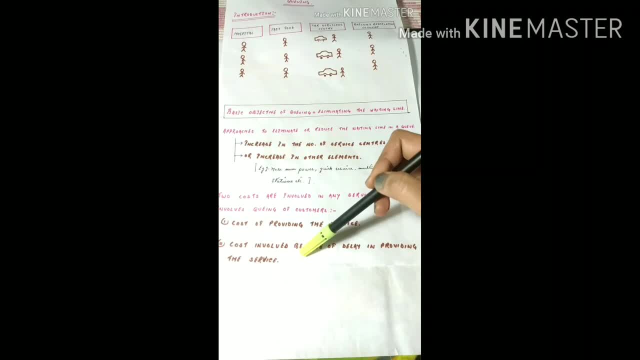 cost involved because of delay in cost involved, because of delay in providing the service that is. this is providing the service that is. this is providing the service that is: this is the cost which is which an organized, the cost which is which an organized, the cost which is which an organized organization has to bear because of the 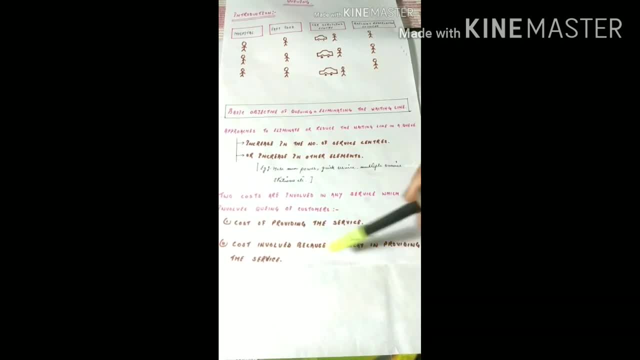 organization has to bear because of the organization has to bear because of the delay, because of the delay created in delay, because of the delay created in delay, because of the delay created in providing the service, that is for providing the service, that is for providing the service that is, for example, yeah, we can, yeah, we can explain. 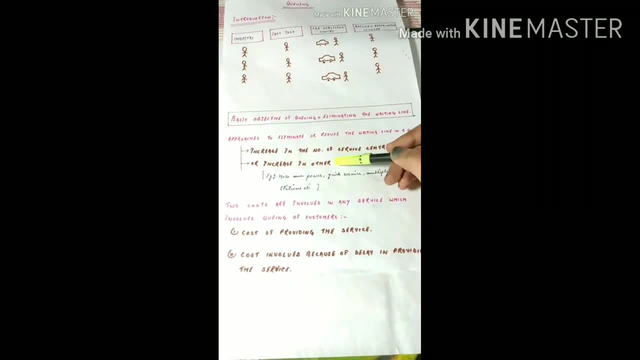 example. yeah, we can. yeah, we can explain example. yeah, we can. yeah, we can explain this point with the help of an example, this point with the help of an example, this point with the help of an example. there is a very common example. yeah, let. there is a very common example. yeah, let. 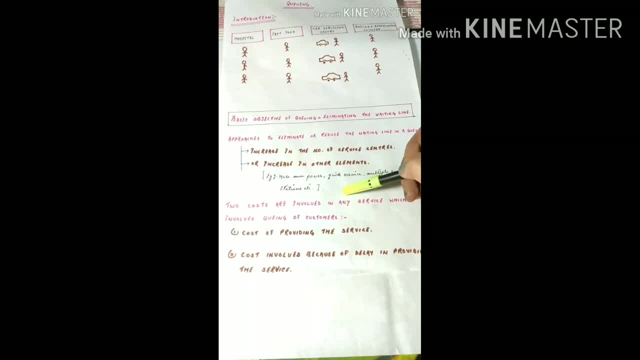 there is a very common example. yeah, let us take this example when we go to a us. take this example when we go to a us. take this example: when we go to a doctor chamber, we are supposed to wait doctor chamber. we are supposed to wait doctor chamber. we are supposed to wait there for our turn to visit the doctor. 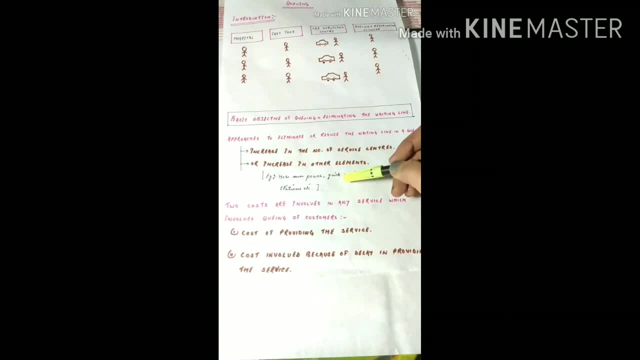 there for our turn to visit the doctor, there for our turn to visit the doctor? okay, so for this purpose, people are okay. so, for this purpose, people are okay. so, for this purpose, people are provided with a waiting hall along with provided with a waiting hall along with. 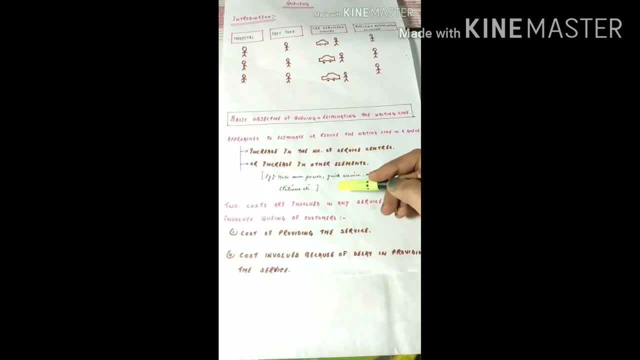 provided with a waiting hall, along with other facilities like lights fans sears, other facilities like lights fans sears, other facilities like lights fans sears, and also, in fact, in some places we do, and also, in fact, in some places we do, and also, in fact, in some places we do find televisions for our entertainment. 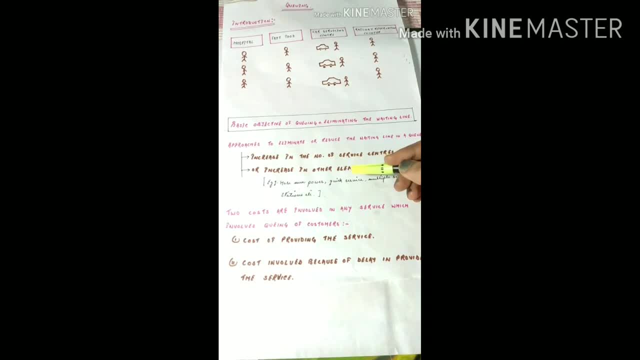 find televisions for our entertainment. find televisions for our entertainment, isn't it? so yeah, this is the cause due, isn't it? so yeah, this is the cause due, isn't it? so yeah, this is the cause. due to the delay in providing the service. so to the delay in providing the service, so 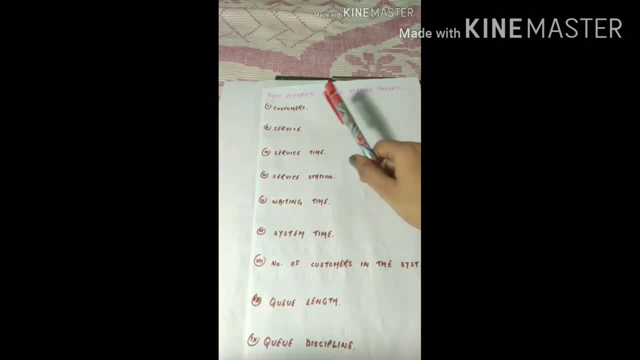 to the delay in providing the service. so now discussing about the basic elements, now discussing about the basic elements, now discussing about the basic elements of curing theory. firstly we have of curing theory. firstly we have of curing theory. firstly we have customers. so customers are regarded as customers. so customers are regarded as. 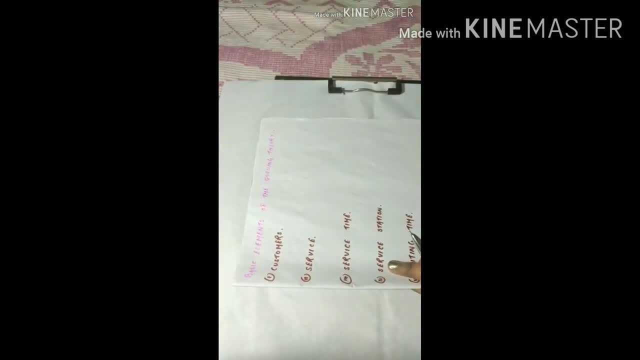 customers. so customers are regarded as the unit arriving for service at the, the unit arriving for service at the, the unit arriving for service at the organization. if we try to depict this organization, if we try to depict this organization, if we try to depict this with the help of a diagram, it will be. 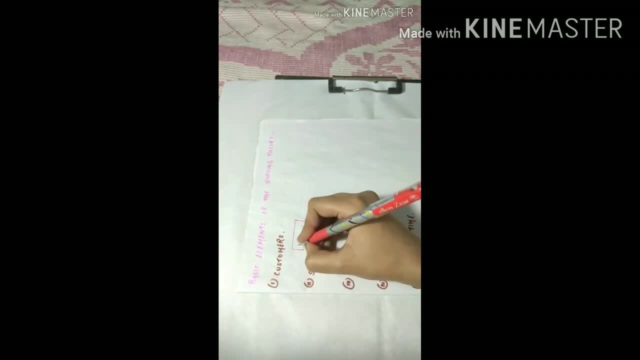 with the help of a diagram. it will be with the help of a diagram. it will be something like this customer which we, something like this customer which we, something like this customer which we will depict it as, will depict it as will depict it as you need, and this be the organization. 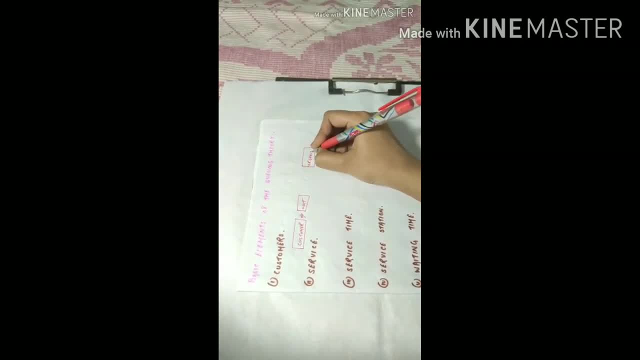 you need and this be the organization you need and this be the organization, and this with the organization so, and this with the organization so, and this with the organization so, customers arriving at the organization, customers arriving at the organization, customers arriving at the organization for service is termed as you need this. 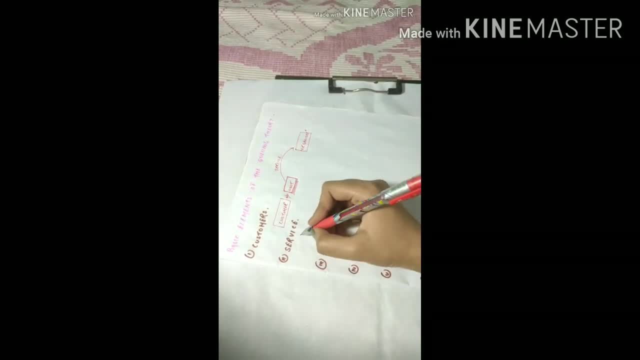 for service is termed as you need this, for service is termed as you need this- other units, then next we have service, so other units, then next we have service, so other units, then next we have service. so service is service is. service is for what the customer has come for. let us 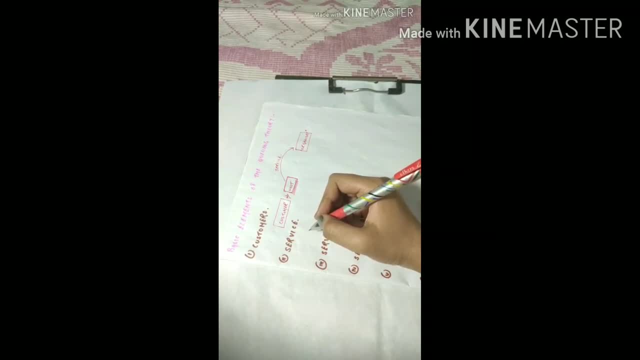 for what the customer has come for. let us for what the customer has come for. let us take an example. so it may be our train. take an example, so it may be our train. take an example, so it may be our train: reservation. it may be a fast-food order. 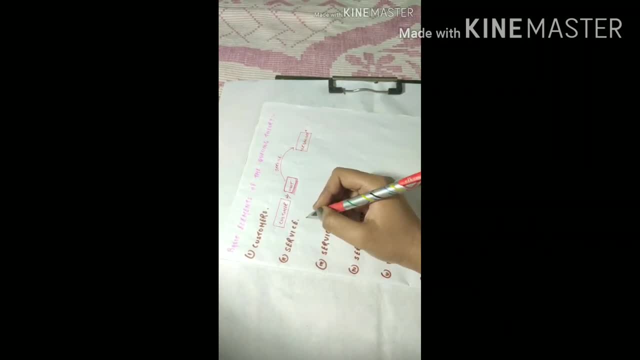 reservation: it may be a fast-food order. reservation: it may be a fast-food order, or it may be a cursor missing whatever, or it may be a cursor missing whatever, or it may be a cursor missing whatever. so if we try to debit this in a diagram, so if we try to debit this in a diagram, 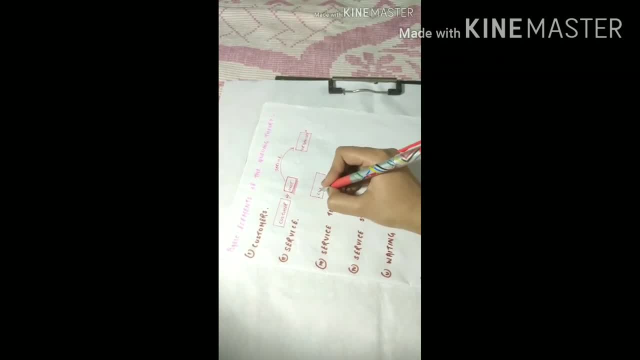 so if we try to debit this in a diagram, so it will be something like this here, so it will be something like this here, so it will be something like this: here will be the customer and for what will be the customer and for what will be the customer and for what, what the customer has come for, that is called. 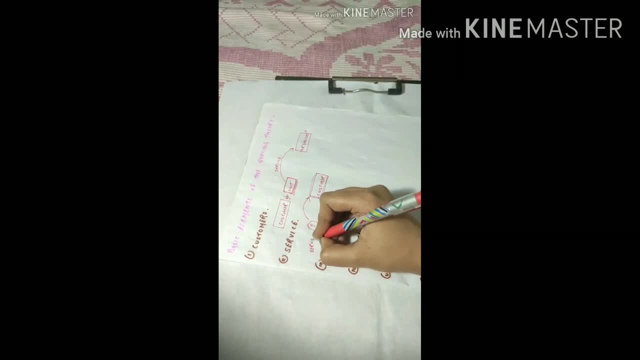 what the customer has come for. that is called what the customer has come for. that is called service, then service time. so it is what the customer has come for, that is called service, then service time. so it is what the customer has come for, that is called service, then service time. so it is the time at which service starts to the 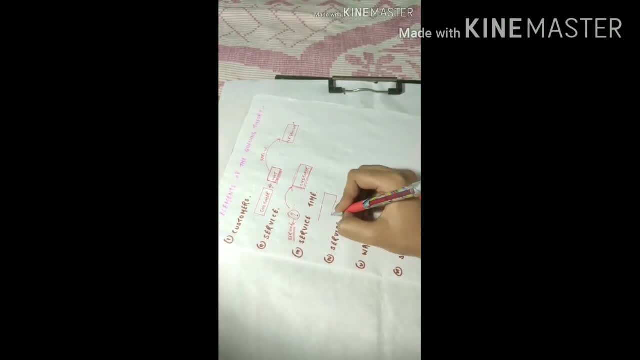 the time at which service starts to the, the time at which service starts to the point at which service ends. so it will point at which service ends, so it will point at which service ends. so it will be something like this, the point at which be something like this, the point at which 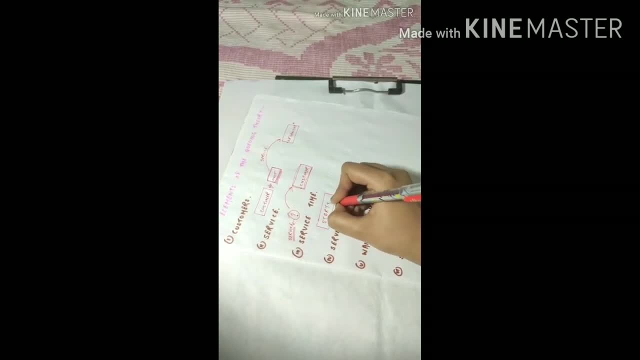 be something like this: the point at which service starts to the point service starts to the point at which service starts to the point service starts to the point at which service starts to the point service starts to the point at which service starts to the point where service ends. so this interval of time 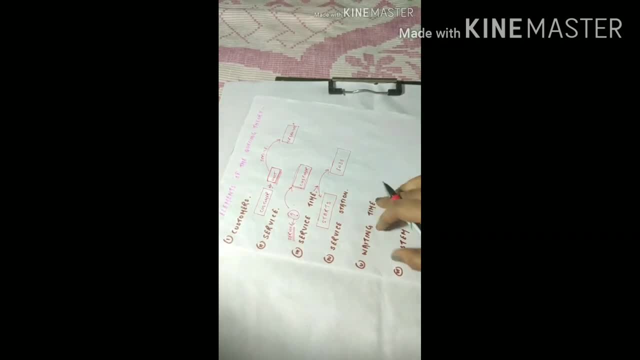 where service ends, so this interval of time where service ends, so this interval of time is termed as service time. so next we is termed as service time, so next we is termed as service time. so next we have the service station, so it is the. have the service station, so it is the. 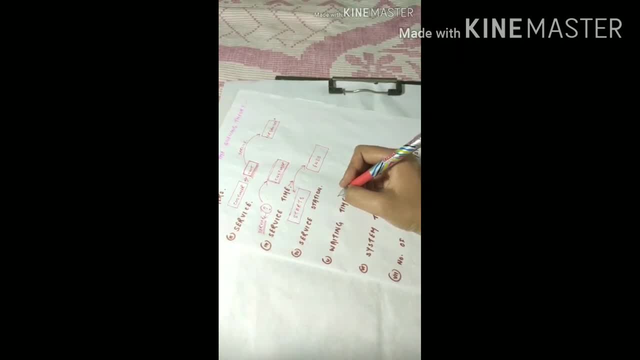 have the service station. so it is the point or place where the service is point, or place where the service is point, or place where the service is provided, for example, in a hospital. it provided, for example, in a hospital. it provided, for example, in a hospital. it would be the reception counter. so if we 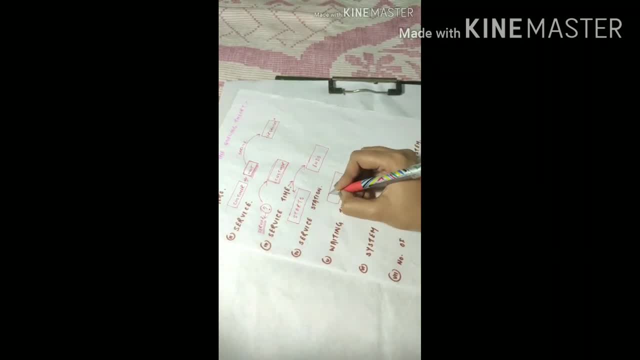 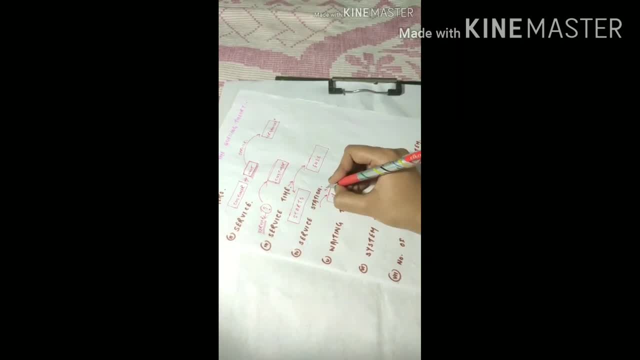 the place or point. so let us write it as the place or point. so let us write it as place where the service is provided, place where the service is provided, place where the service is provided, provided, the place where service is provided, the place where service is provided, the place where service is provided, is service station. then then, 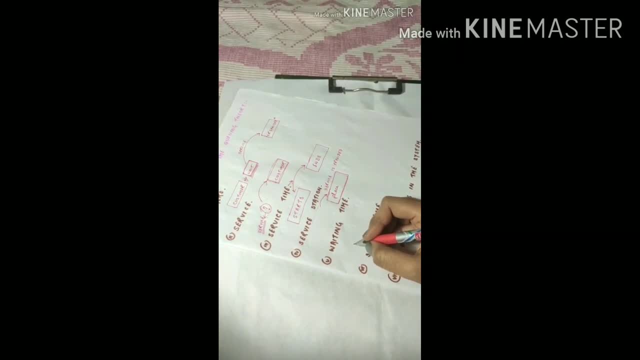 provided is service station, then then provided is service station, then then then next we have is the waiting time. so then next we have is the waiting time. so then next we have is the waiting time. so this is the time the customer waits. this is the time the customer waits. 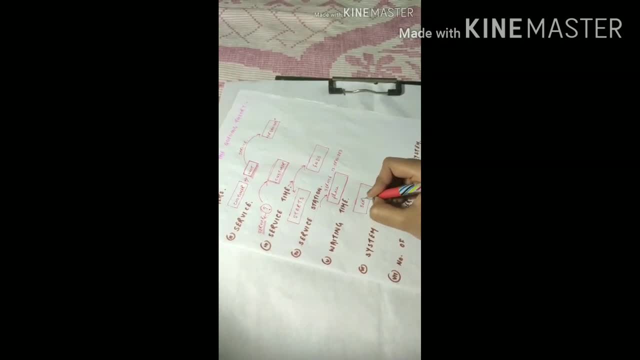 this is the time the customer waits before getting the service, before getting the service, before getting the service. so this is the service. the time the so this is the service. the time the so this is the service. the time the customer waits before getting the service. customer waits before getting the service. 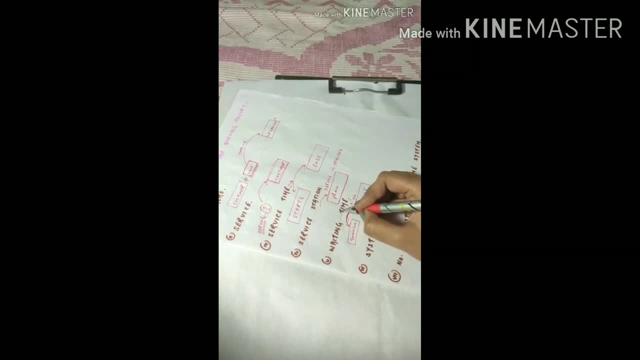 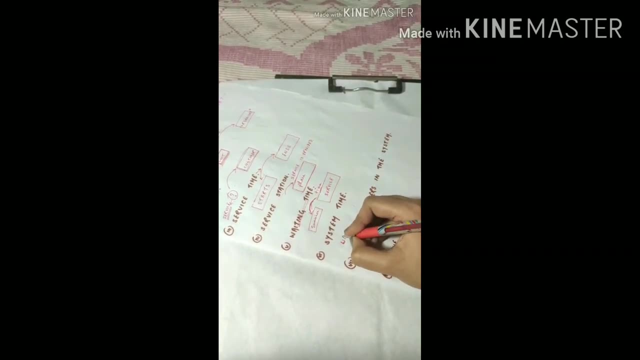 customer waits before getting the service. so this time, this time is called. so this time, this time is called. so this time, this time is called waiting time. the next is a system time waiting time. the next is a system time waiting time. the next is a system time. so it is the sum of waiting time. 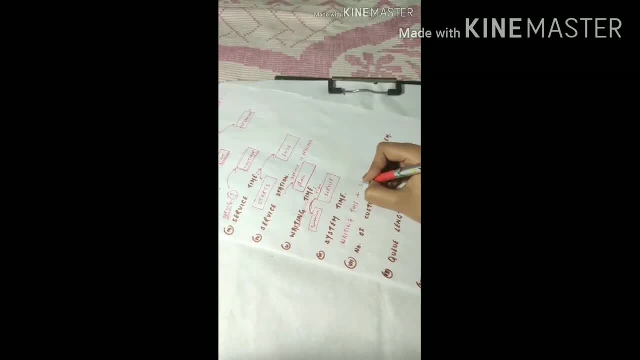 so it is the sum of waiting time. so it is the sum of waiting time, waiting time plus service time, the sum of waiting time plus service time, the sum of waiting time plus service time. the sum of this two is termed as system time next. this two is termed as system time next. 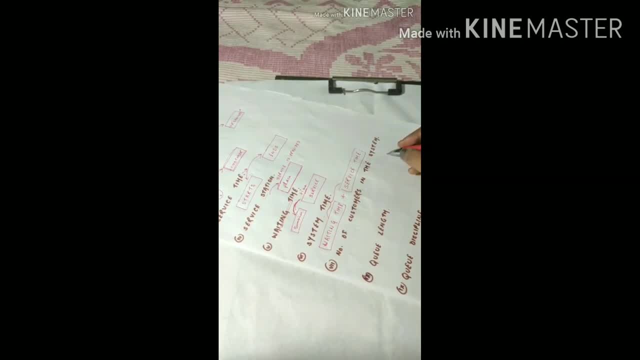 this two is termed as system time. next, we have is number of customers in the. we have is number of customers in the. we have is number of customers in the system. so this is equal to the number of system. so this is equal to the number of system. so this is equal to the number of customers waiting in the queue, plus. 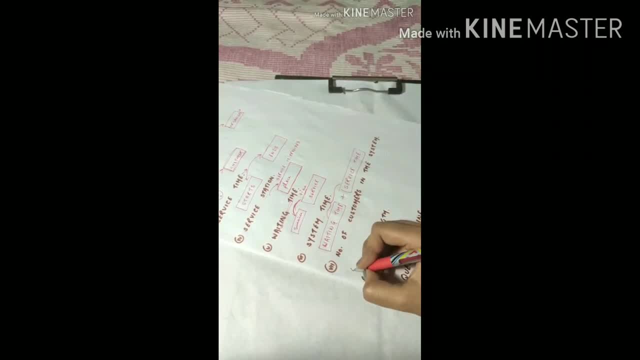 customers waiting in the queue plus customers waiting in the queue, plus number of customers getting the service, number of customers getting the service, number of customers getting the service. so number of customers waiting in the queue plus the customers waiting in the queue, plus the customers waiting in the queue, plus the customers who are getting the service. I hope you. 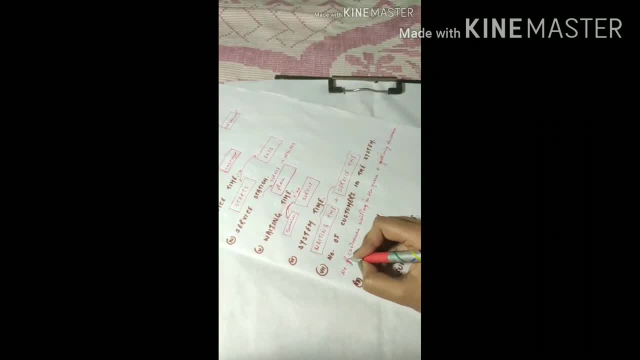 who are getting the service. I hope you who are getting the service. I hope you are understanding my handwriting. the next are understanding my handwriting. the next are understanding my handwriting. the next that we have is queue length, so it is. that we have is queue length, so it is. 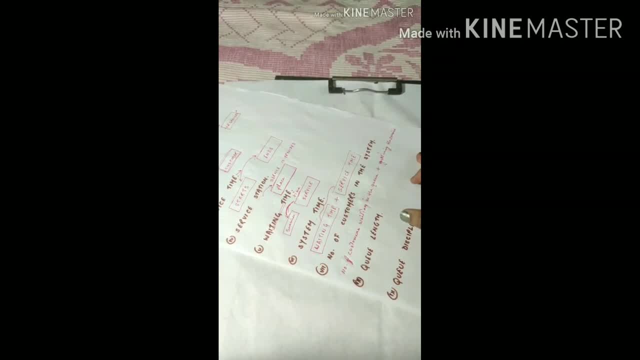 that we have is queue length. so it is nothing but the number of customers, nothing but the number of customers, nothing but the number of customers waiting for service in the queue, and then waiting for service in the queue, and then waiting for service in the queue, and then, lastly, we have the queue discipline. so 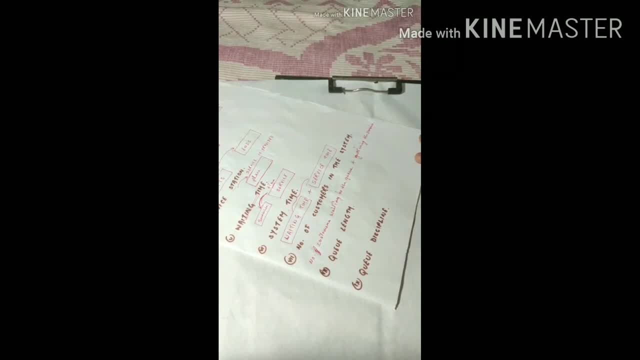 lastly, we have the queue discipline. so, lastly, we have the queue discipline, so it is that pattern according to which it is that pattern according to which it is that pattern according to which the customers are picked up from the queue. the customers are picked up from the queue. 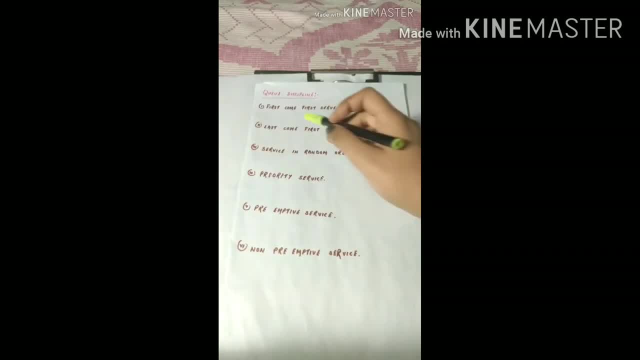 the customers are picked up from the queue and, and they are provided service so to and. and they are provided service so to, and. and they are provided service. so to analyze the queue discipline. we have the analyze the queue discipline. we have the analyze the queue discipline. we have the following behaviors: the first that we 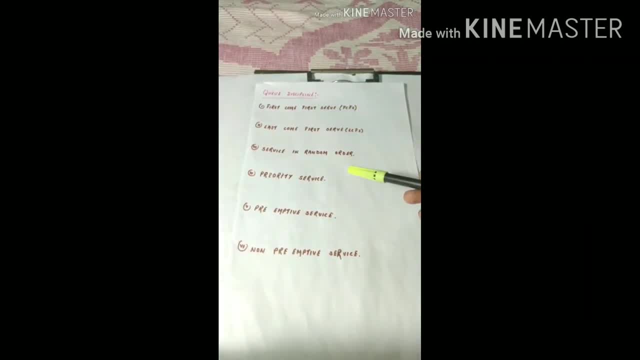 following behaviors, the first that we following behaviors, the first that we have is the first come first serve. so have is the first come first serve. so have is the first come first serve. so this is the most commonly used queue. this is the most commonly used queue. this is the most commonly used queue discipline, which gives first priority to: 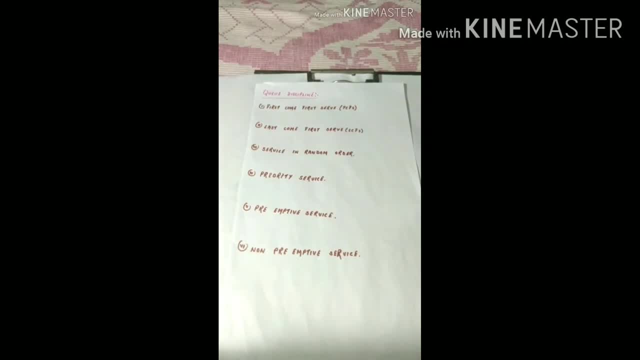 discipline, which gives first priority to discipline, which gives first priority to those units or customers that have come, those units or customers that have come, those units or customers that have come first. so next that we have is the last first. so next that we have is the last. 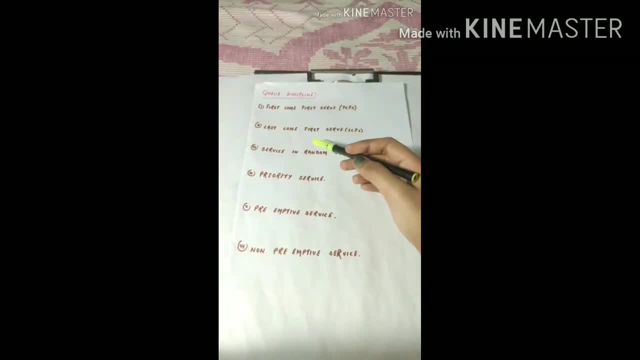 first. so next that we have is the last come first serve. so here units which come first serve. so here units which come first serve. so here units which come last are processed first. so let us come first serve. so here units which come last are processed first. so let us. 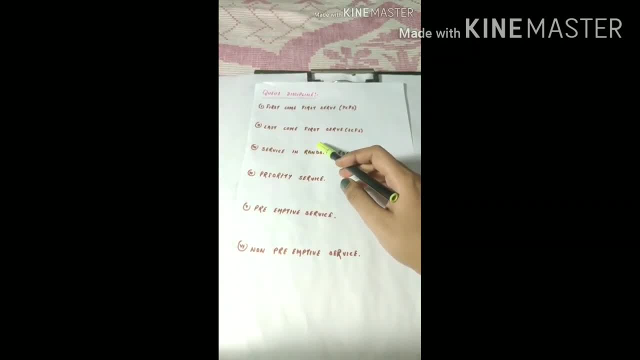 come first serve. so here, units which come last are processed first. so let us take an example for when we go for. take an example for when we go for. take an example for when we go for purchasing medicines, then we generally purchasing medicines, then we generally purchasing medicines, then we generally purchase those medicines which have. 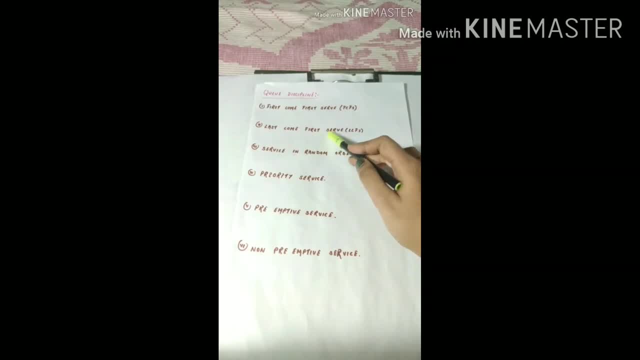 purchase those medicines which have, purchase those medicines which have manufacturing date latest, so that manufacturing date latest, so that manufacturing date latest, so that example suits this condition well and example suits this condition well, and example suits this condition well. and then next we have is service in random. 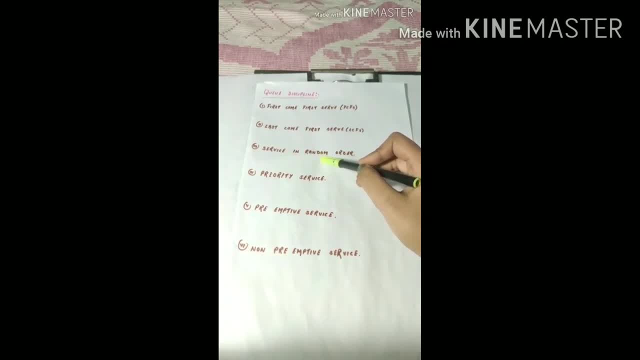 then next we have is service in random. then next we have is service in random. here units are selected from the waiting here. units are selected from the waiting here. units are selected from the waiting hall in random basis. so there is no hall in random basis, so there is no. 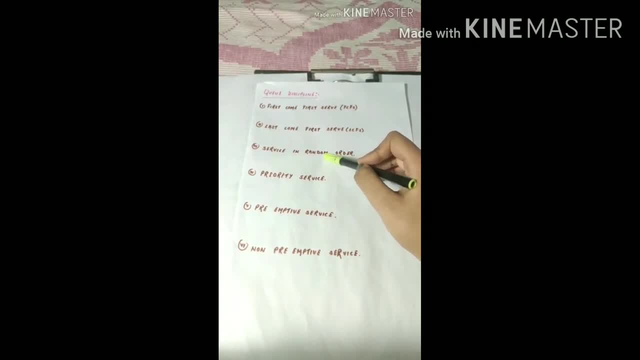 hall in random basis. so there is no well-defined procedure for selection, so well-defined procedure for selection, so well-defined procedure for selection. so in this, in this behavior, there is no in this, in this behavior, there is no in this. in this behavior, there is no well-defined procedure for selection. so 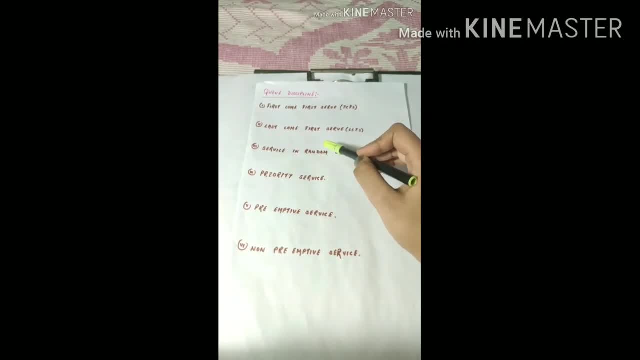 well-defined procedure for selection, so well-defined procedure for selection. so so customers are selected in random for so customers are selected in random for so customers are selected in random for service. so next that we have is priority service. so next that we have is priority service. so next that we have is priority service. in this discipline, units are: 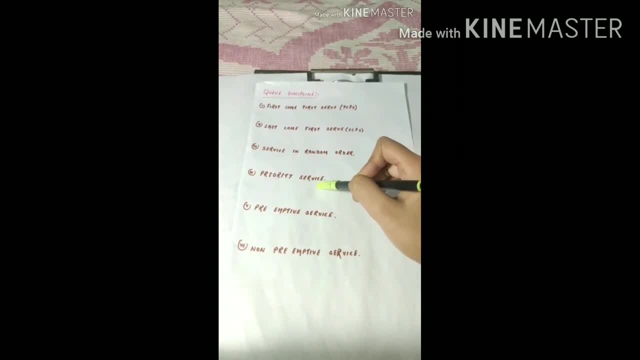 service. in this discipline, units are service. in this discipline, units are first selected on the basis of some first selected, on the basis of some first selected on the basis of some priority rule. that that's why it is priority rule. that that's why it is priority rule. that that's why it is named as priority service. so let us take 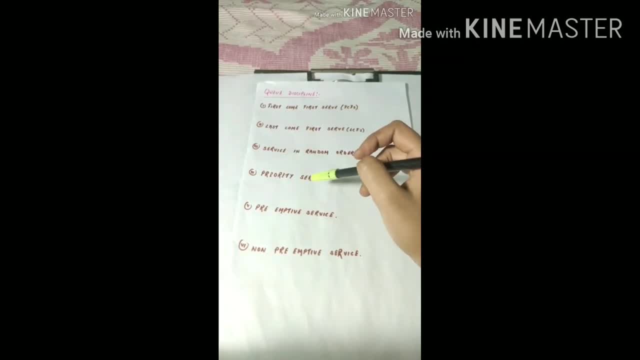 named as priority service, so let us take named as priority service. so let us take an example to here that, in case of an example to here that, in case of an example to here that, in case of hospitals, those patients are looked hospitals, those patients are looked hospitals, those patients are looked immediately, whose condition is critical. 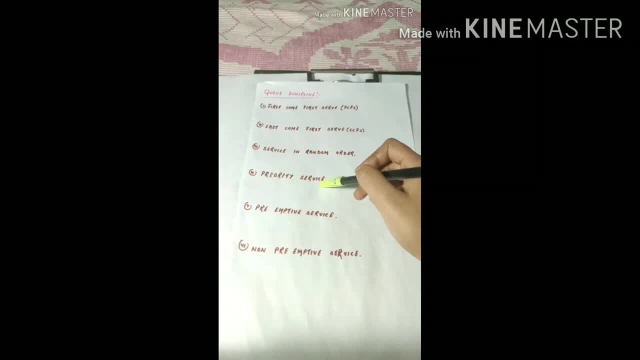 immediately whose condition is critical, immediately whose condition is critical and rest of the patients are looked, and rest of the patients are looked, and rest of the patients are looked afterwards, so that example suits this afterwards, so that example suits this afterwards, so that example suits this condition. and then we have the preemptive. 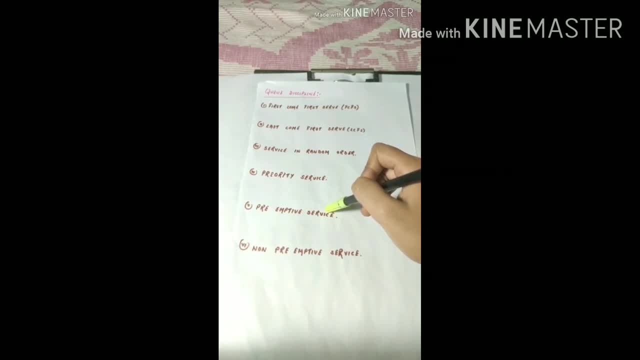 condition, and then we have the preemptive condition and then we have the preemptive service. so in this type you need with service, so in this type you need with service. so in this type you need with high priority are attended first, even high priority are attended first, even. 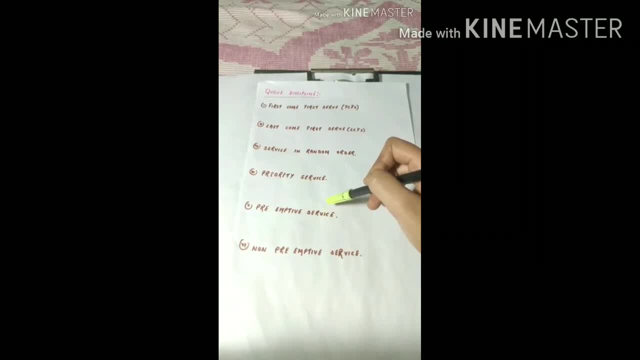 high priority are attended first, even though low priority are already though low priority are already though low priority are already receiving the service. so so their receiving the service. so so their receiving the service. so so their services stop temporarily, and the services stop temporarily, and the services stop temporarily and the service is given to the high priority. 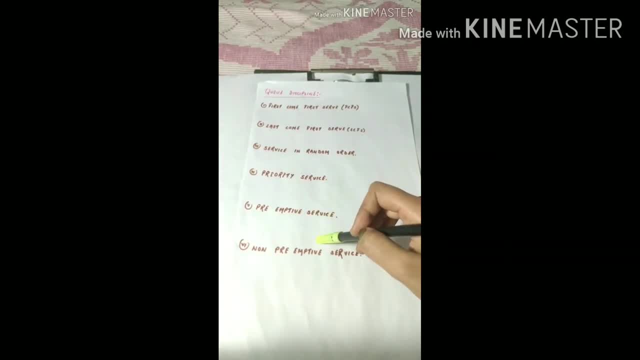 service is given to the high priority, service is given to the high priority customers. so next we have the customers. so next we have the customers. so next we have the non-preemptive priority. so in this case, non-preemptive priority. so in this case, non-preemptive priority. so in this case, high priority unit goes ahead in the queue. high priority unit goes ahead in the queue. high priority unit goes ahead in the queue, but still have to wait until the but still have to wait until the but still have to wait until the service of the car, until the current service of the car, until the current. 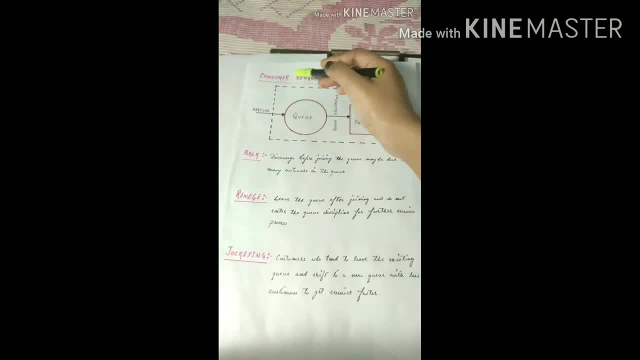 service of the car until the current service is not completed. now proceeding service is not completed now proceeding service is not completed. now proceeding to the consumer behavior. as in the to the consumer behavior. as in the to the consumer behavior, as in the diagram, we can see that a person arrives. 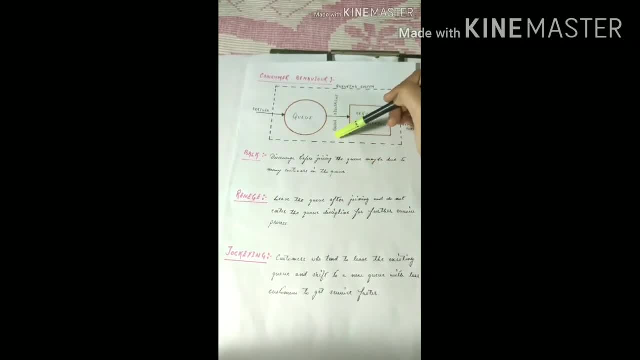 diagram. we can see that a person arrives diagram. we can see that a person arrives at a particular service station. he joins at a particular service station. he joins at a particular service station, he joins the queue in a particular queue, the queue in a particular queue, the queue in a particular queue, discipline, and then he gets the service. 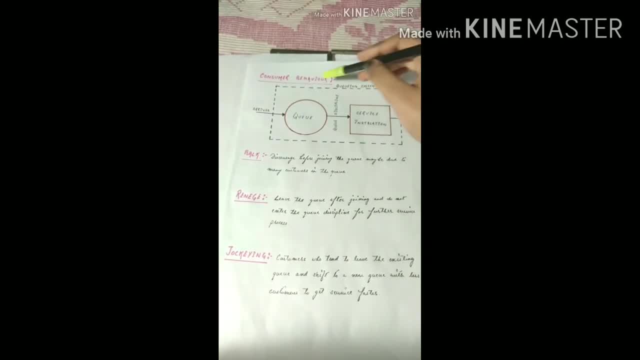 discipline, and then he gets the service discipline and then he gets the service, and then he departs from the service and then he departs from the service and then he departs from the service station. this system is called queuing station. this system is called queuing. 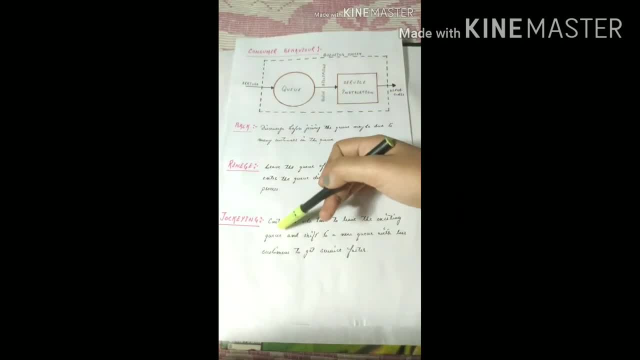 station. this system is called queuing system now. so now we will discuss about system now. so now we will discuss about system now. so now we will discuss about three types of customers. firstly, we have three types of customers. firstly, we have three types of customers. firstly, we have the bulk, so this type of customers get 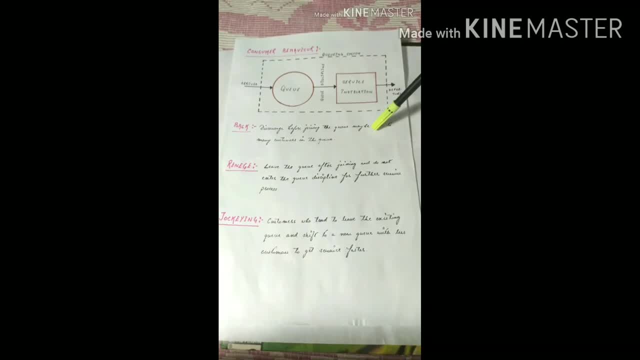 the bulk, so this type of customers get the bulk. so this type of customers get discouraged even before joining the queue. discouraged even before joining the queue, discouraged even before joining the queue. and this may be due to many numbers of. and this may be due to many numbers of. 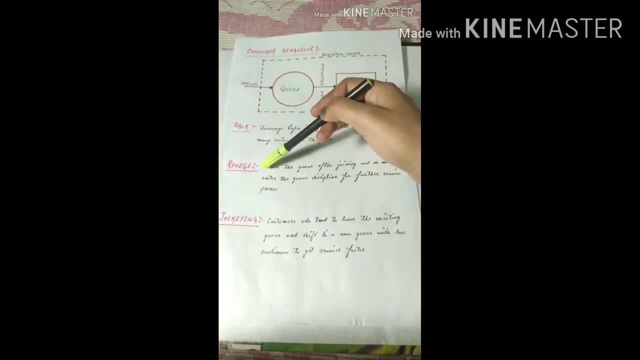 and this may be due to many numbers of customers in the queue. the next thing we customers in the queue, the next thing we customers in the queue, the next thing: we have drainage. so this type of customers have drainage. so this type of customers have drainage. so this type of customers leave. take you after joining and do not. 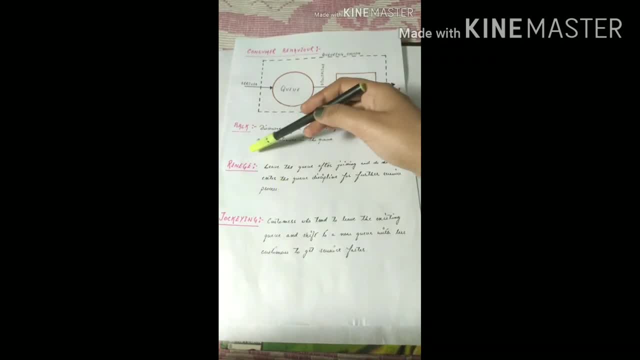 leave. take you after joining and do not leave. take you after joining and do not enter the queue discipline for further enter the queue discipline for further enter the queue discipline for further service process. so this type of service process, so this type of service process, so this type of customers, can be considered far more. 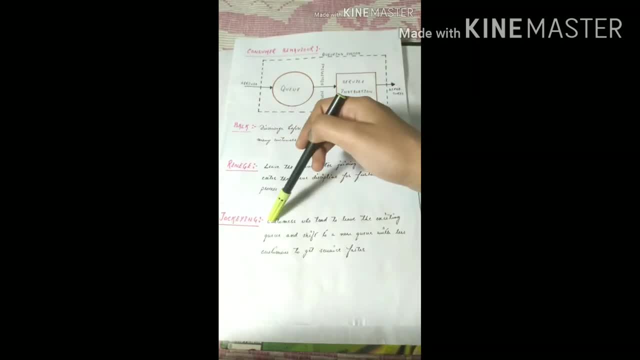 customers can be considered far more customers can be considered far more patient than this type of customers, patient than this type of customers, patient than this type of customers. lastly, we have the jockeying this type. lastly, we have the jockeying this type. lastly, we have the jockeying this type of customers who tend to leave the 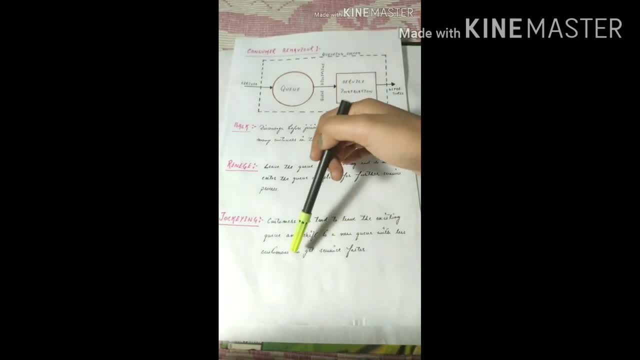 of customers who tend to leave the. of customers who tend to leave the existing queue and shift to a new queue- existing queue and shift to a new queue- existing queue and shift to a new queue with less customers. to get service with less customers. to get service with less customers. to get service faster. so this is it for this video. 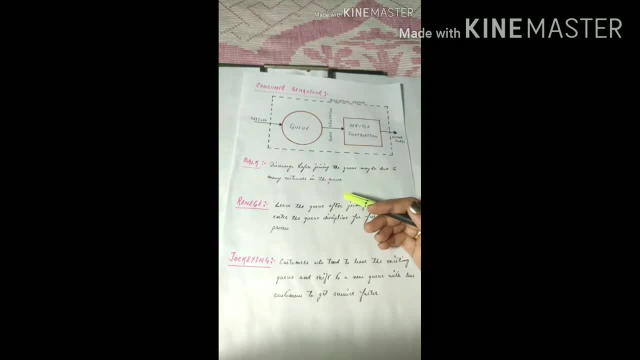 faster. so this is it for this video: faster, so this is it for this video. please watch our next video to learn. please watch our next video to learn. please watch our next video to learn more concepts of queuing theory and do more concepts of queuing theory and do.